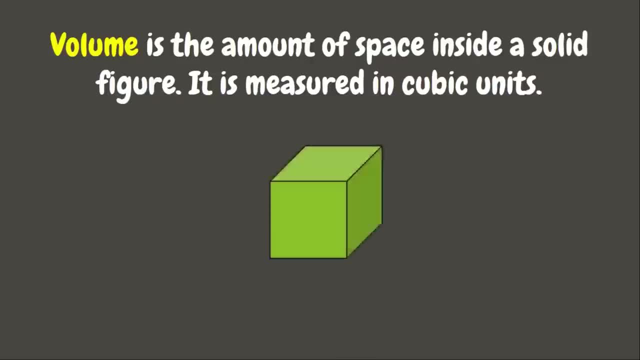 in volume. it is measured in cubic units. Cubic unit is a cube whose sides measure 1 unit. If each side measures 1 cm, it will be called 1 cubic cm. If they are 1 meter, the volume would be 1 cubic meter. 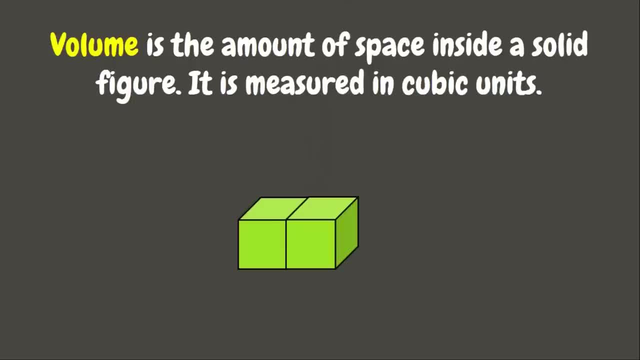 Now, if we have two cubes whose sides measure 1 unit, the volume would be 2 cubic units. If we add one, that would be 3 cubic units. And let's say we have three more, That would be 6 cubic units. Here we can see that we have formed a rectangular prism whose height 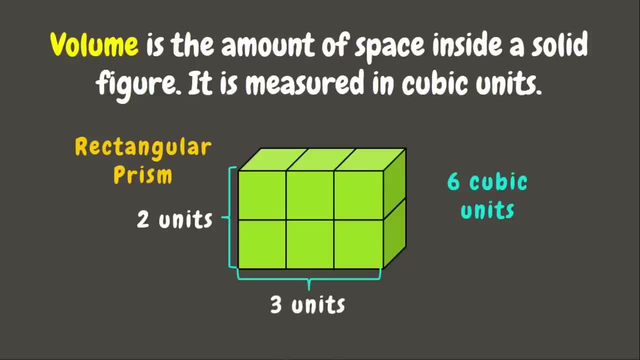 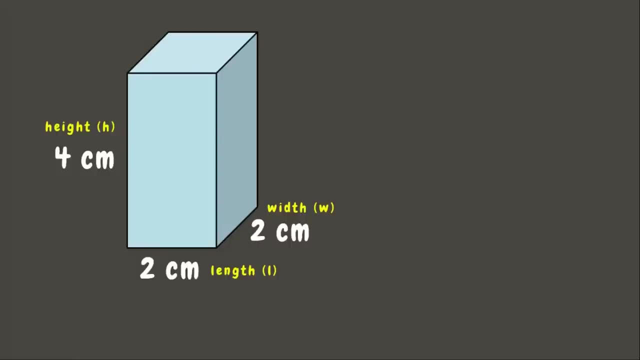 measures 2 units, length 3 units and the width 1 unit. We can determine the volume of a figure by counting the number of cubic units that can fit inside it. Now let's try and go back to our problem. Now let's try to make some cubic units using the dimension of this figure, Here the rectangular. 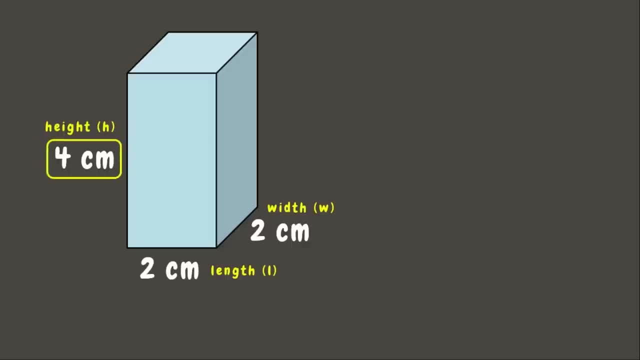 prism has the height of 4 cm. It means it has 4: 1 cm, So that would be 1,, 2,, 3, and 4.. Now for the length. it has 2 cm, So that would be 1,, 2,, 3, and 4.. Now for the length. 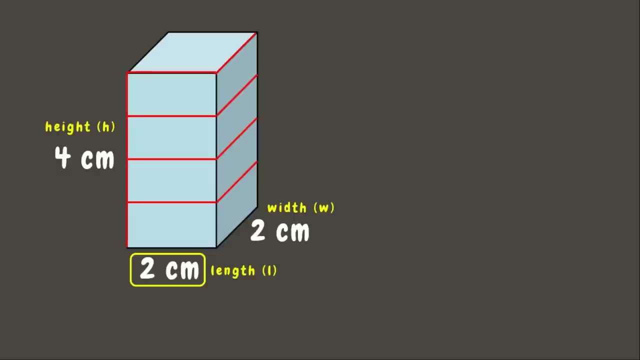 it has 2 cm, So that would be 1,, 2,, 3, and 4.. Now for the length: it has 2 cm, So that would be 2 cm. So that would be 2 cm, 1 and 2.. 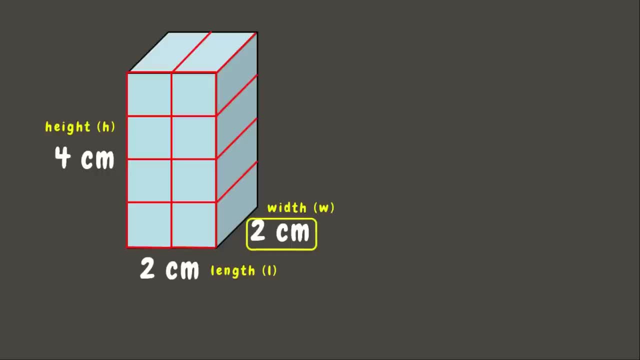 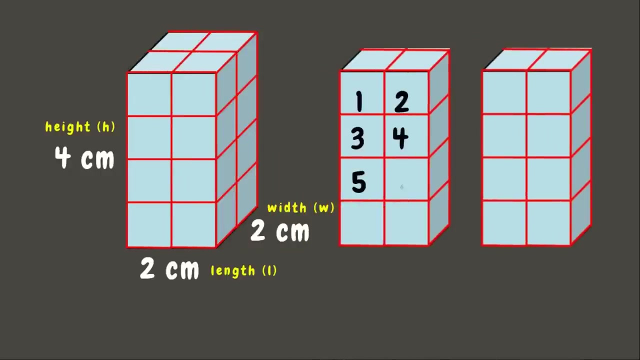 And also for its width. It has 2 cm, So that would be 1 and 2.. Now we have formed some cubic units. Now let us count them, we have 16 cubic units, or 16 cubic centimeters, and that's the volume of this prism. now we can observe. 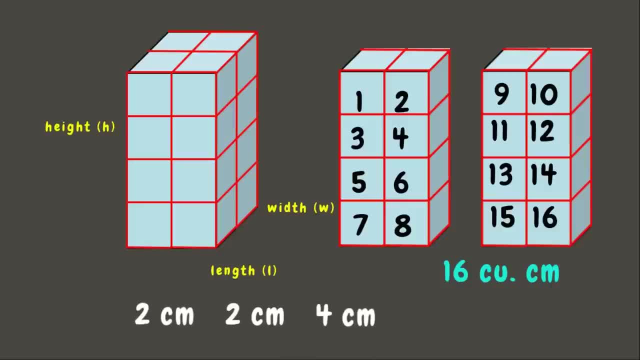 that if we multiply 2 centimeters to 2 centimeters to 4 centimeters, we will get the volume 16 cubic centimeters. this means that to get the volume of a prism we can simply multiply the length to its width, to its height, or that will be length times width times height. 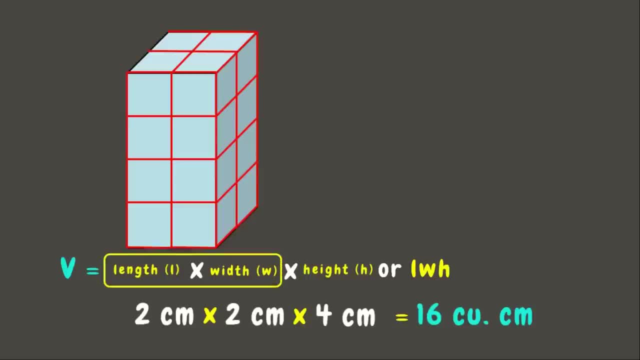 also, we can observe that the length times the width is the area of the base. therefore, we can also say that to get its volume, we can multiply the area of the base to its height, so that will be area of the base times the height. now, as we can see, we are multiplying three. 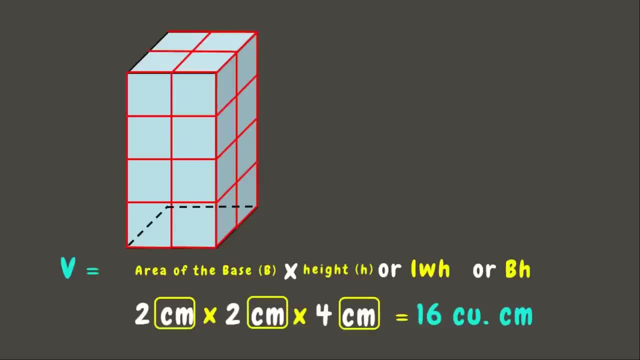 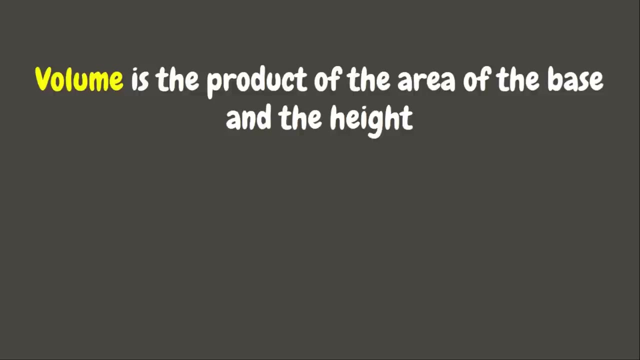 dimensions. therefore, we can also write the answer as 16 cubic centimeters, with 3 as the exponent. wonderful. now we learned that the volume is the product of the area of the base and the height, so we can make a formula as: b equals area of the base times the height. wonderful. 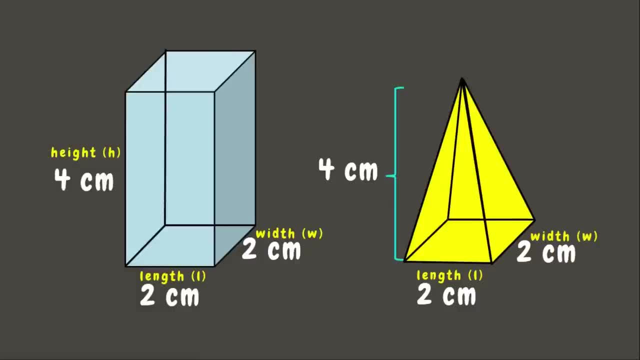 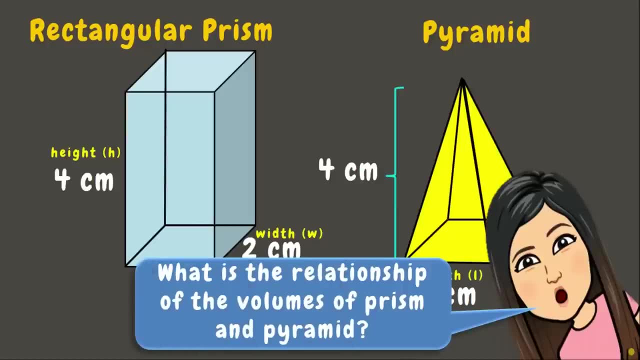 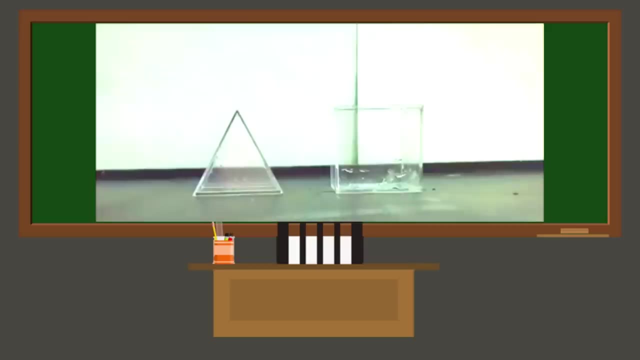 now let's take a look at these two figures. we have a rectangular prism and a pyramid with the same height and base. now let's determine the relationship of the volumes of prism and pyramid using an experiment. here: the prism and the pyramid has the same height and base. 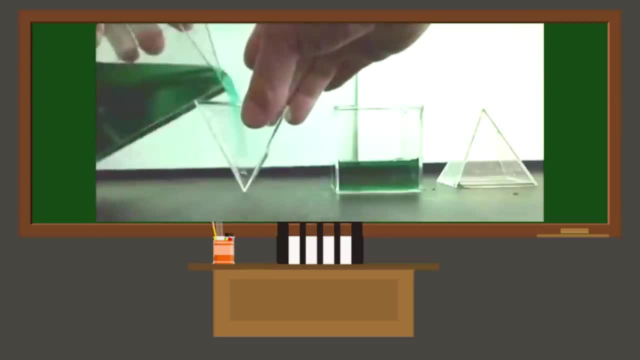 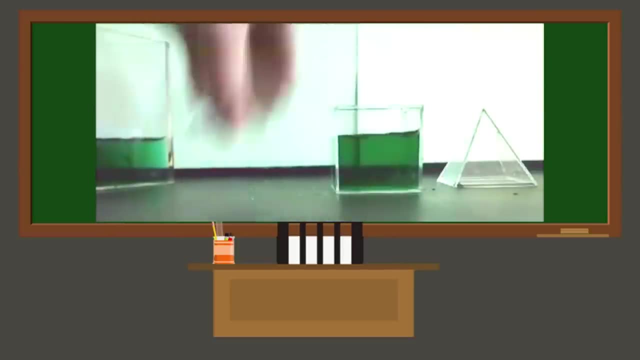 therefore, i have to describe one experiment with a total difference. something like lakes Peradd regulate necrotism. here the justement: we believe that the area where we have dirt at the surface of a wall is not protected by one genius. so this experiment has a horizontal slope, namely that the soil 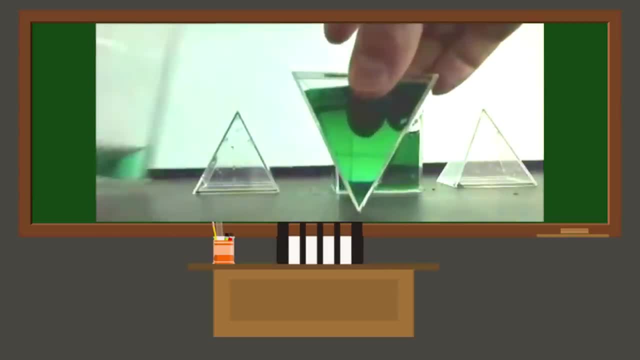 in which we are seeing it has an sixteen degree angle and on the surface of the brain we have an equation where absolute double squared hallway. everything we can see here is just a these areas filter index. so here we haveip. duplicate value will be equal to to CAR塊. 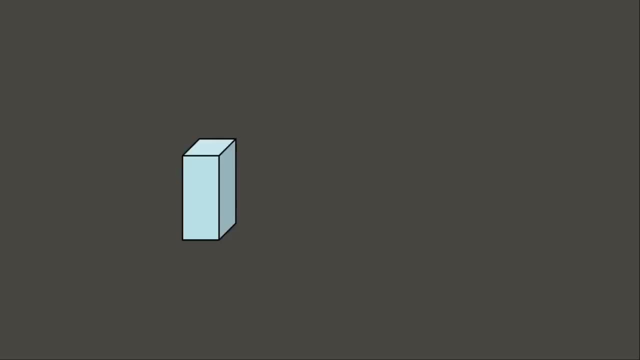 09d. as per the equation expression in agency we have q's, in this case, the professionals build orders. there are also expressions to be to b s s of these values and values you want to43. We learned that one rectangular prism is equal to three pyramids, considering that they have the same height and base. 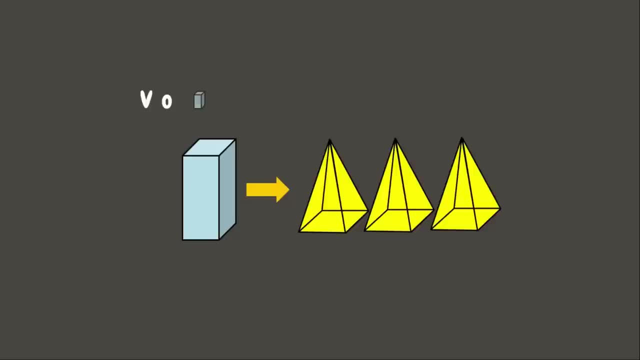 Therefore we can say that the volume of the pyramid is equal to one-third of the volume of the rectangular prism. So the formula for the pyramid's volume is one-third times the length times the width times the height, or length times width times the height, divided by three. 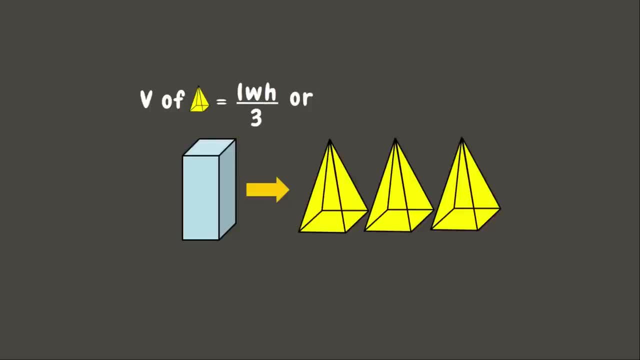 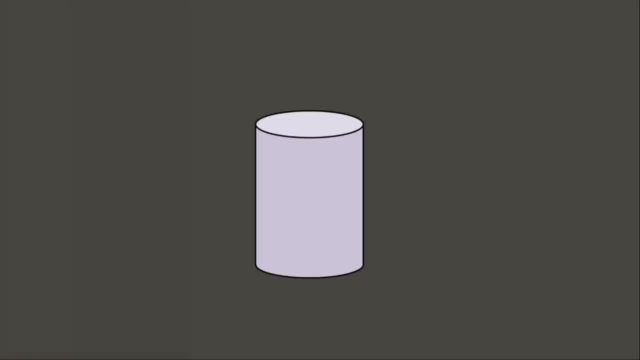 Or we could also say that the volume of the pyramid would be one-third of the area of the base times the height. Awesome. Next up, we have here a cylinder. Again. since we know the volume is equal to the area of the base times the height, let's try to make a formula for the volume of cylinder. 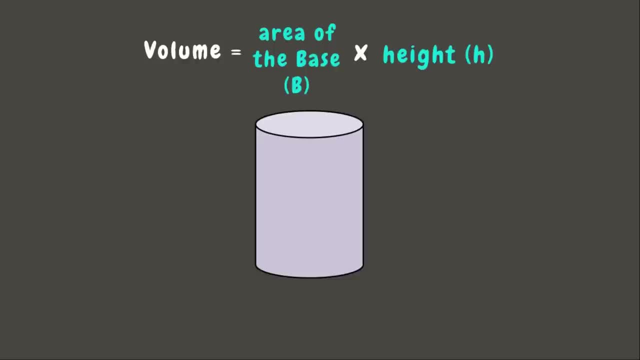 First, let's identify its base. Since it has circular base, we can say that The area of the base will be the area of the circle, which is pi r-squared. Therefore, that will be. volume of the cylinder is equal to pi r-squared times the height. 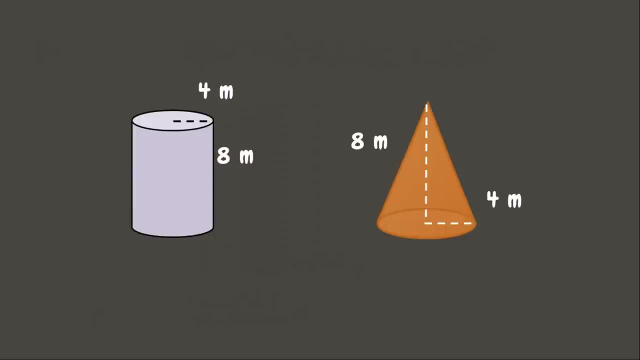 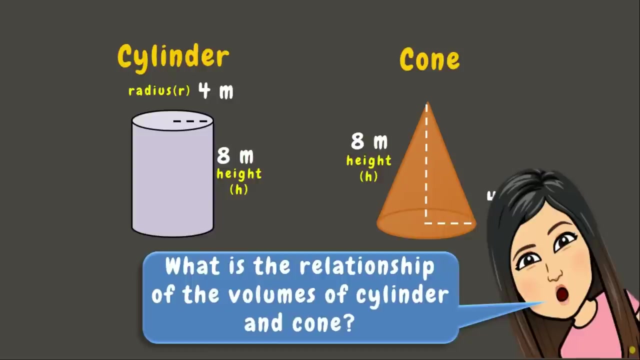 Great job. Now let's take a look at these two figures. We have here a cylinder and a cone with the same height, base and radius. Now let's determine the relationship of the volumes of the cylinder and cone using an experiment. 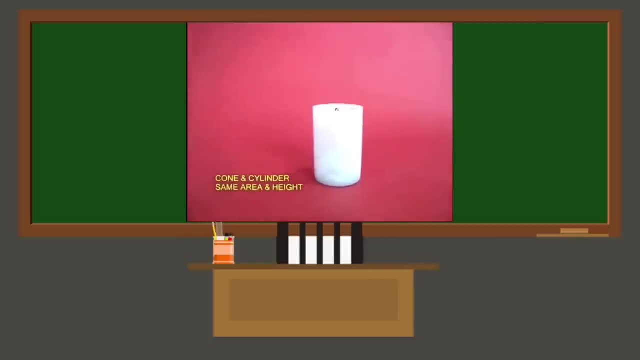 Here we can see that the cylinder and the cone has the same height and base. This is the same height as the base and the cylinder. The volume is one-third times the area of the base, times the height, which is pi r-squared. 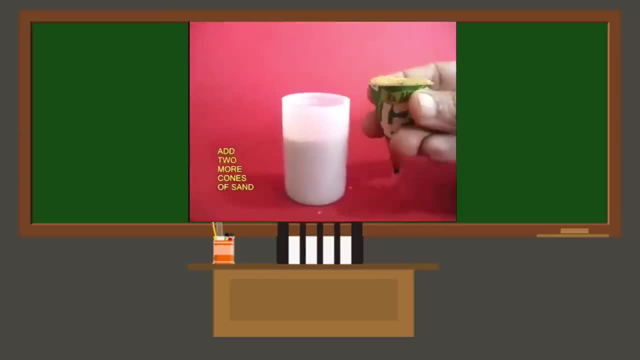 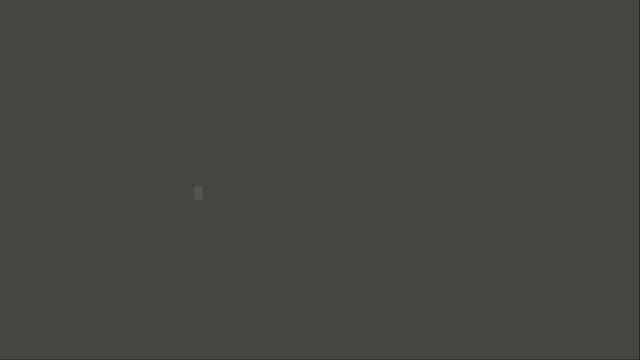 And this is the same volume as the base of the cylinder. Let's try saying that: Esta es una cinta de un cinta de un cinta. From the experiment we learned that one cylinder is equal to three cones, considering that they have the same height and base. 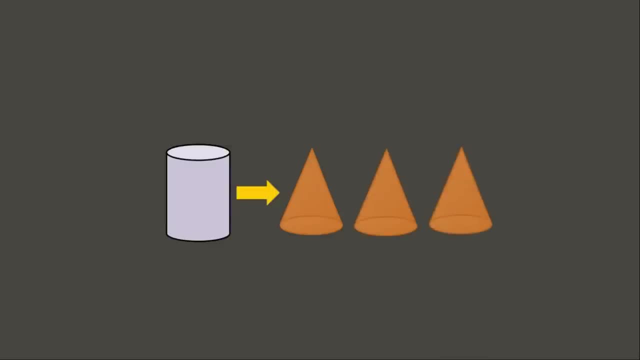 Therefore we can say that the volume of the cone is one-third of the volume of the cylinder. So the formula for the cone's volume is one-third times pi? r-squared h, or pi? r-squared h divided by three. Great job. 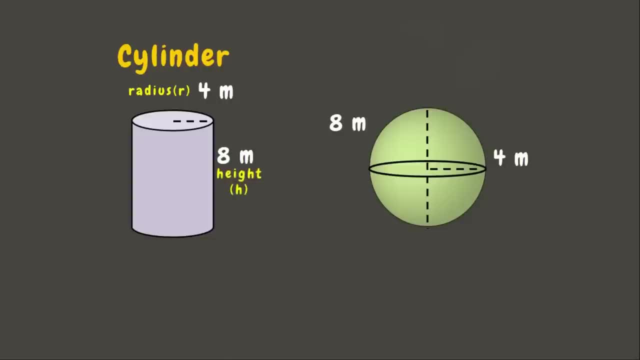 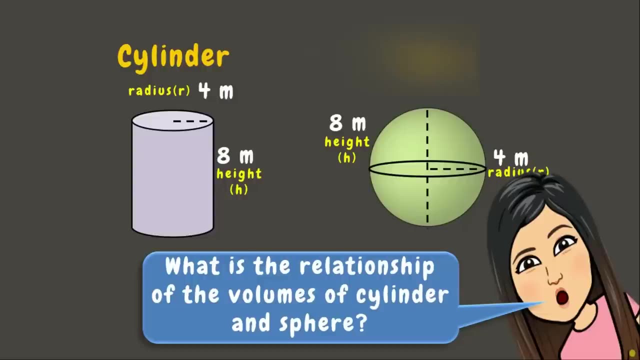 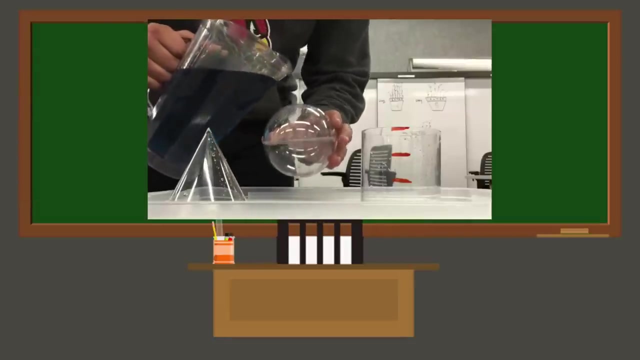 Last one. we have a cylinder and a sphere with the same height and radius. Now let's determine the relationship of the volumes of the cylinder and sphere using an experiment. In this experiment, the sphere and the cylinder has the same height and radius.